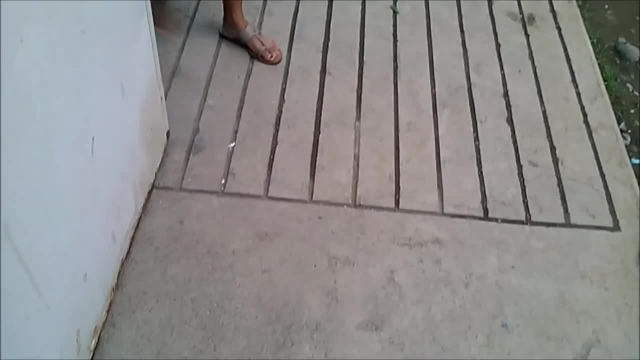 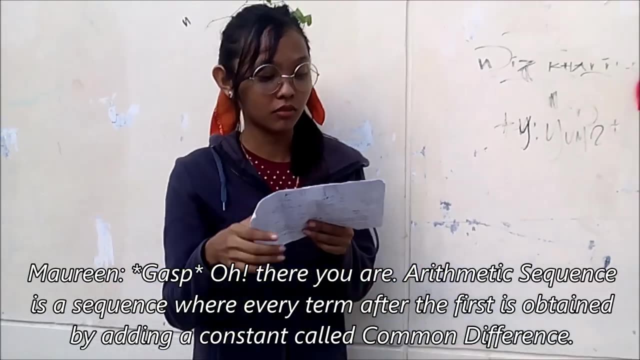 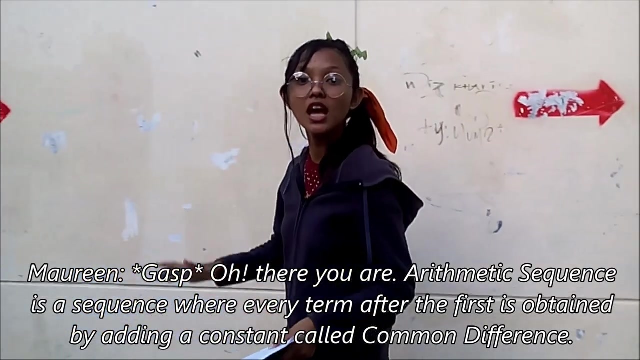 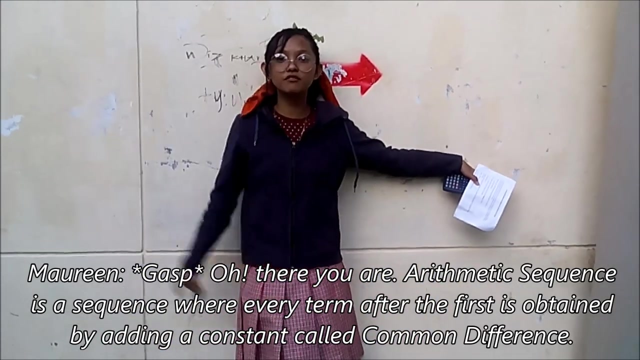 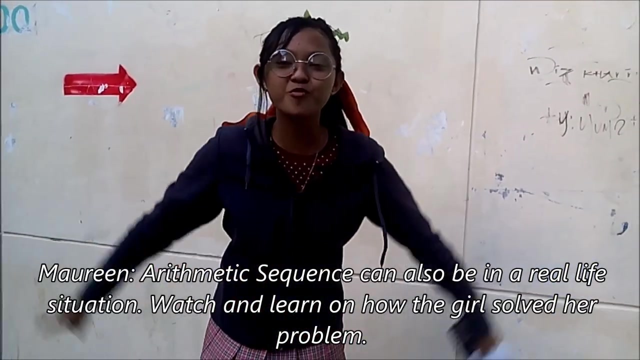 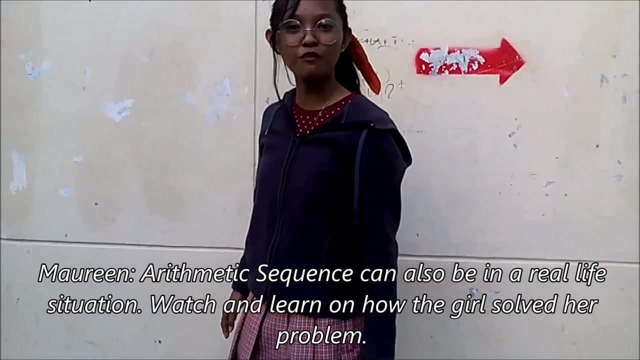 Oh, there you are. Arithmetic sequence is a sequence where every term of the first is obtained, by which a constant called a common difference. Arithmetic sequence can also be a real-life situation. Watch and learn on how the girl she solved her problem. 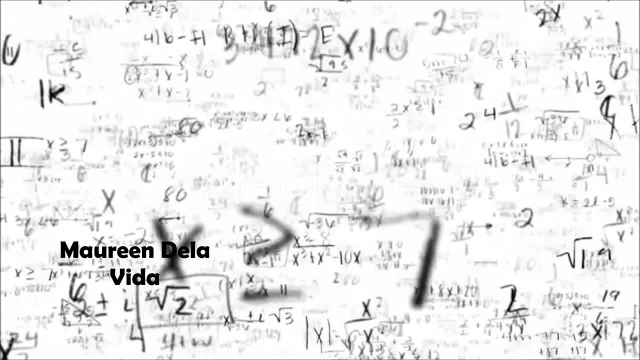 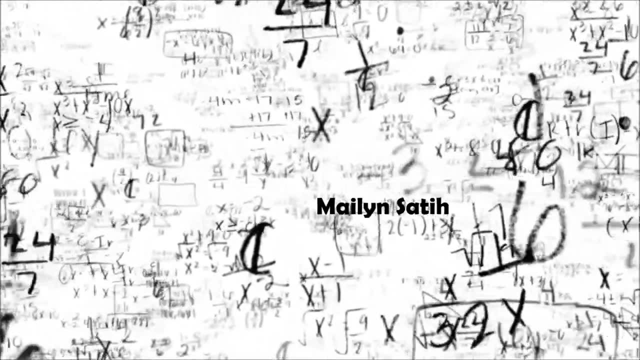 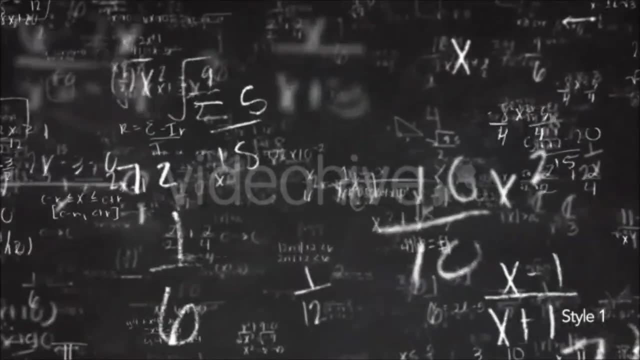 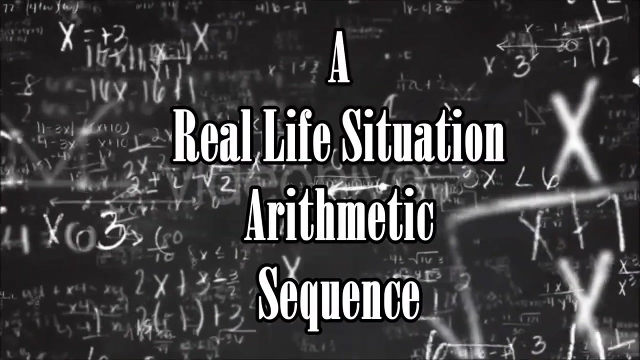 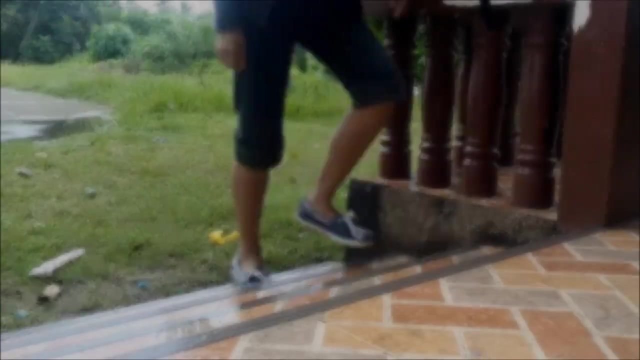 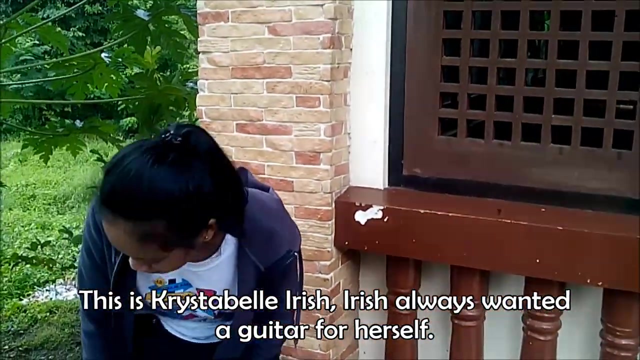 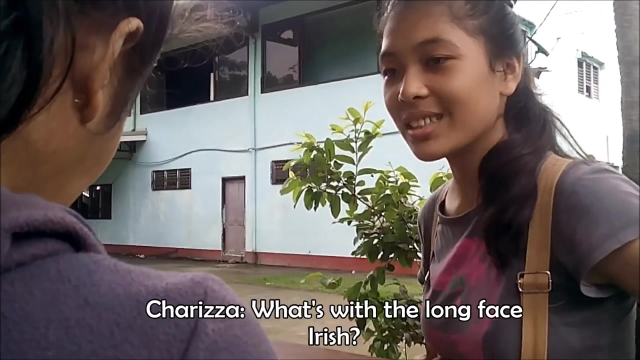 Arithmetic sequence can also be a real-life situation. Watch and learn on how the girl she solved her problem. This is Christabel Irish. Irish always wanted a guitar for herself. What's been the wrong place, Irish? I wish I had a guitar, but my mind is not looking right. 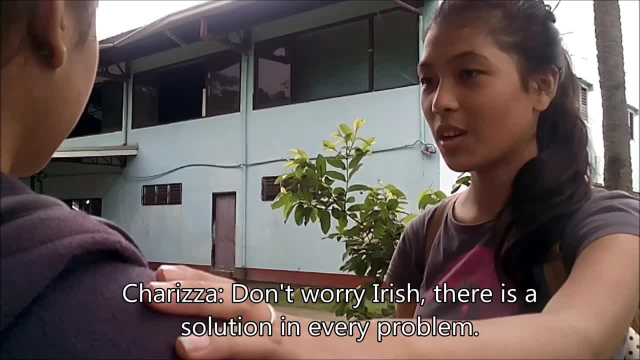 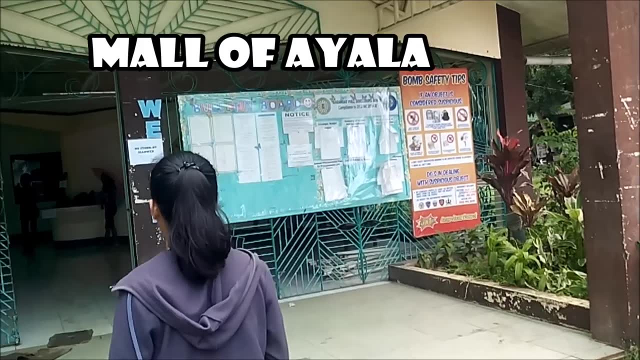 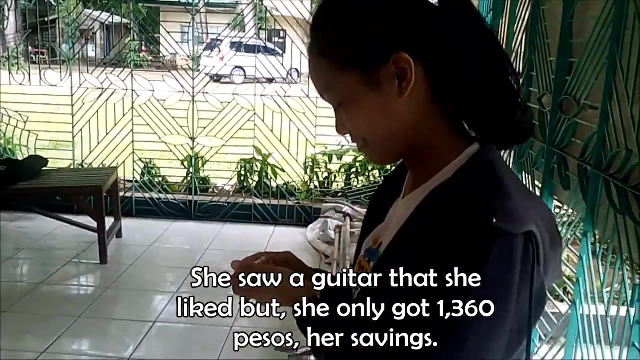 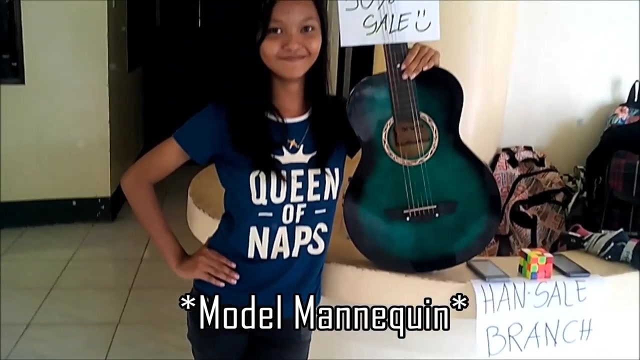 Stop worrying. There's a solution in every problem. Okay, One day, While she was walking, she saw a guitar that she liked, But she only got 1360 pesos. her savings, Oh my god, my favorite guitar. 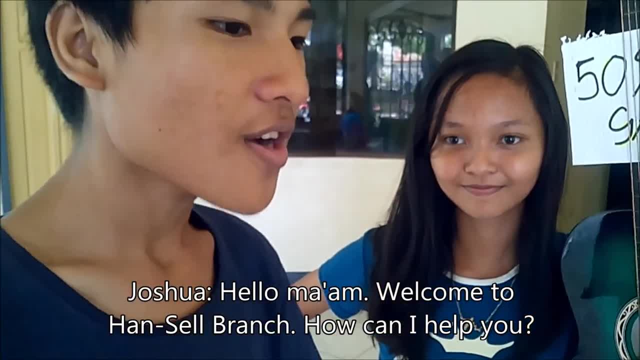 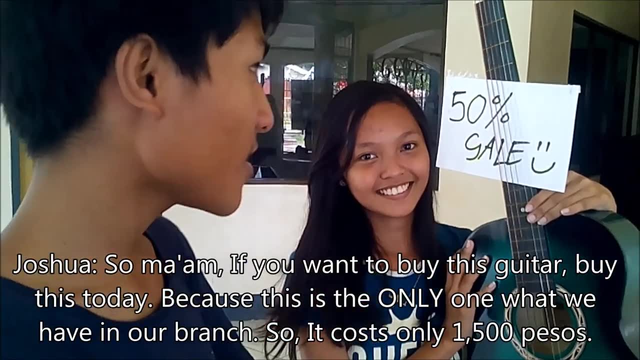 Hello, mom, Welcome to Argyle Ranch. How are you? How much do you need Five. So, mom, you want to buy this guitar. Buy this today, because that is the only one that we have in our yard. 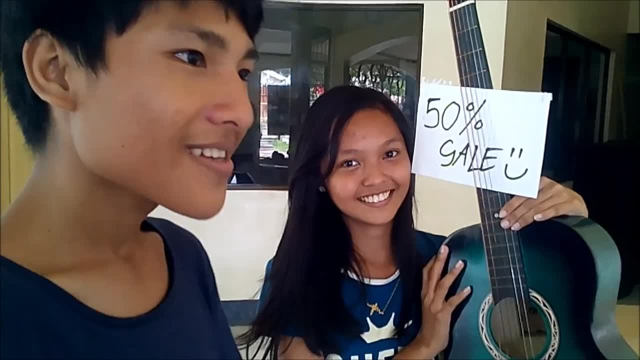 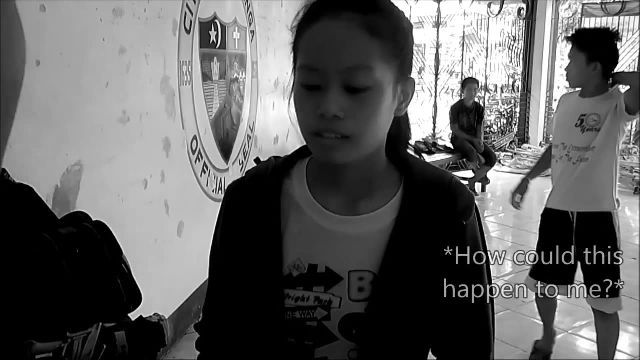 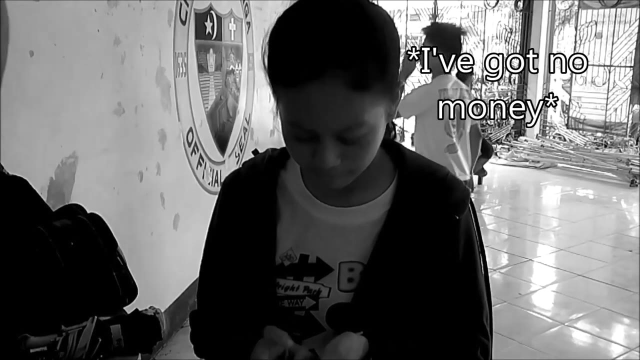 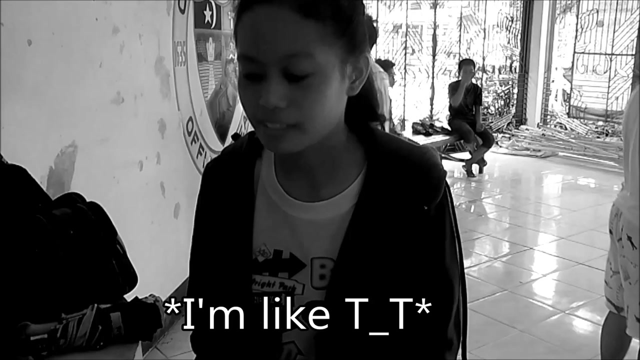 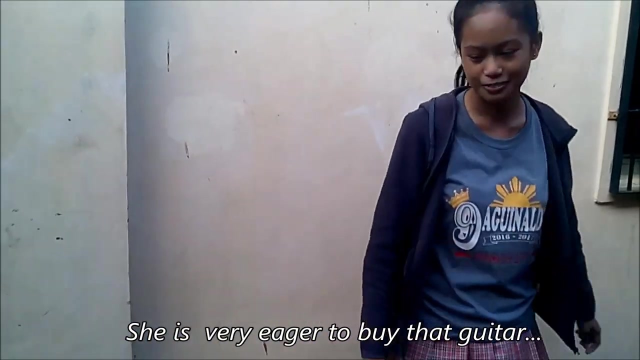 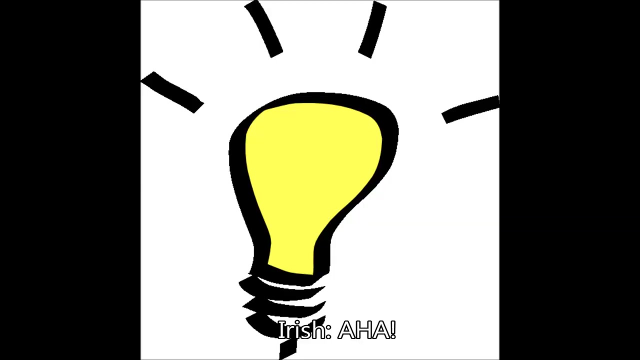 Oh my god, But it costs only 1500.. In case you cannot understand, in case you cannot, She is very eager to buy that guitar, So she came up with an idea. Aha, I know I'll start to work tomorrow so that I can buy the guitar for you. 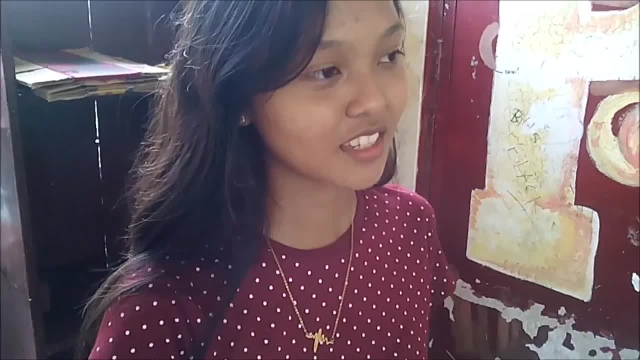 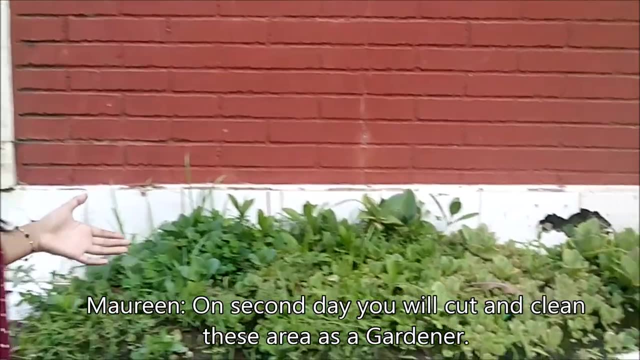 So do you want to work for me? Yes, ma'am. On first day, you will clean this as a street sweeper. On second day, you will cut and clean this area as a garden. On third day, you will clean this window as clean as my place. 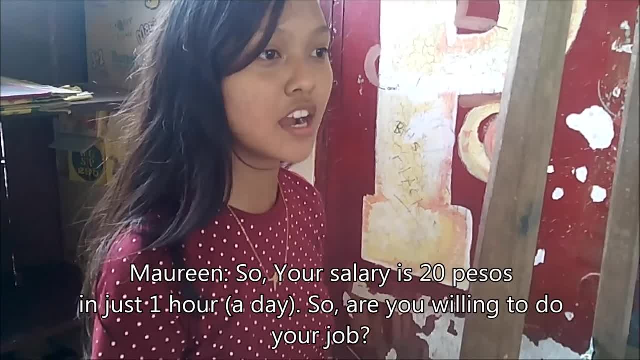 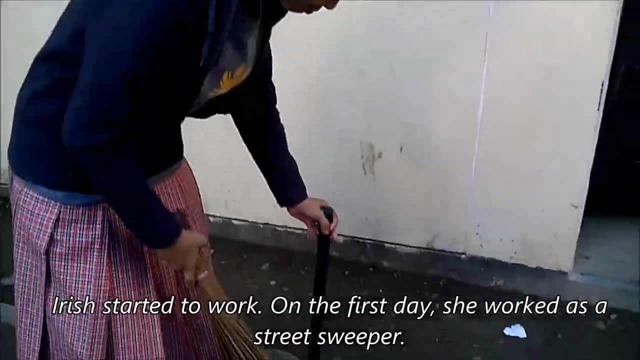 So your salary is 20 pesos, just one hour. So are you willing to do your job? Yes, ma'am, So we are clear now. So Irish started to work. On the first day she worked As a street sweeper. 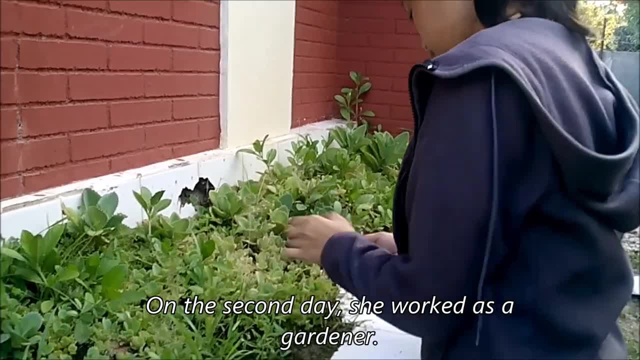 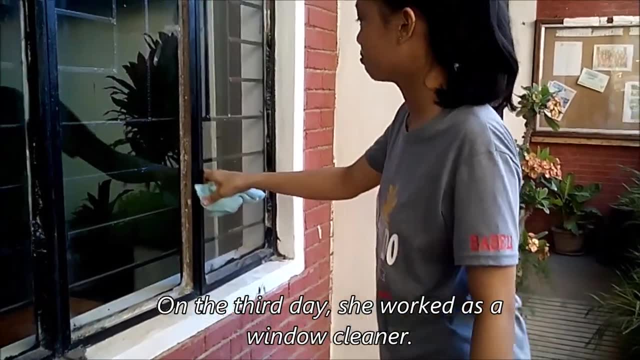 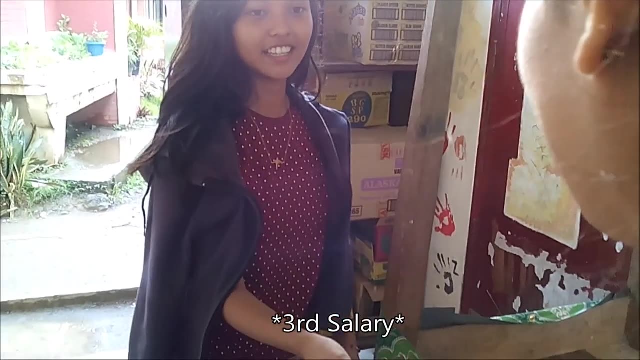 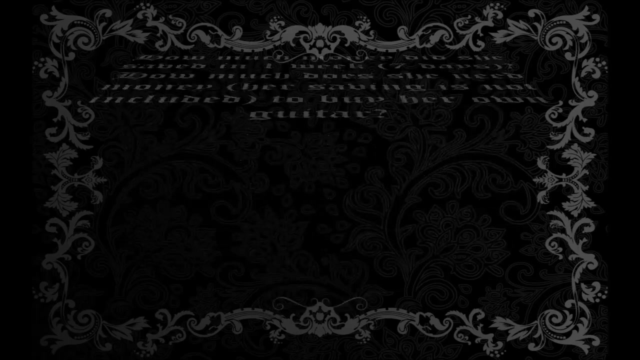 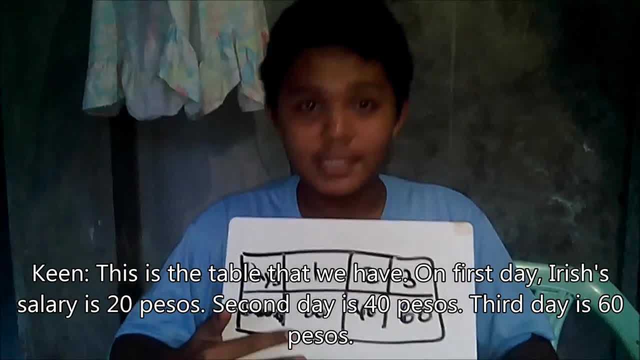 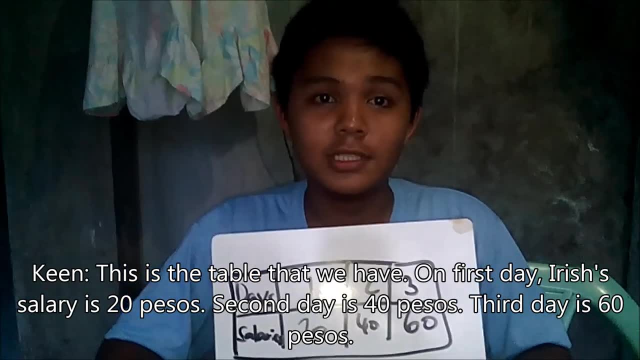 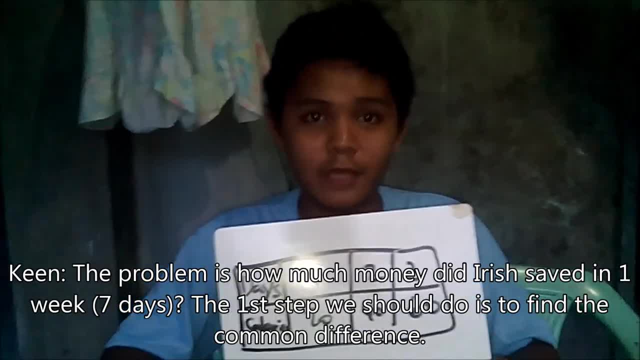 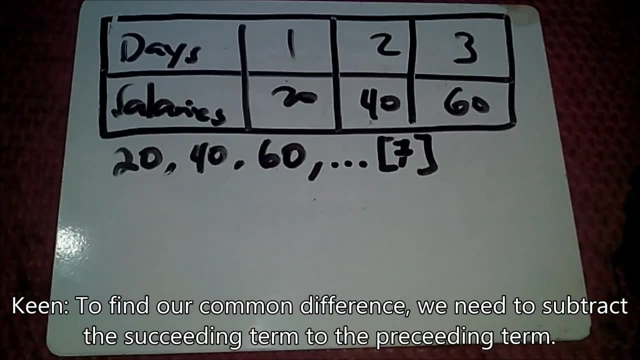 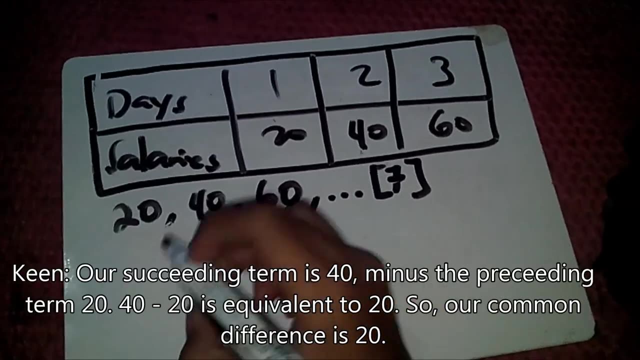 The problem is: how much money did Irish save in one week? The first step we should do is to find the common difference. So to find our common difference, we need to subtract the succeeding term to the preceding term. Okay, Our succeeding term is 40 minus our preceding term 20..